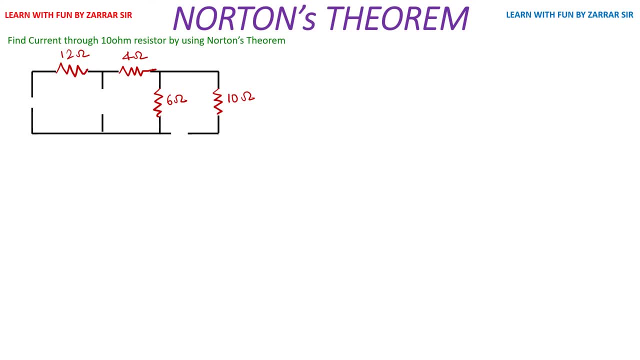 okay, write one. let's write one more resistance over here, that's 2 ohm. okay, and let's take two voltages. I'll take 1 volt as 20 volt over here and let's take some higher value over here of voltage. I'll assume it to be 40 volt, okay. 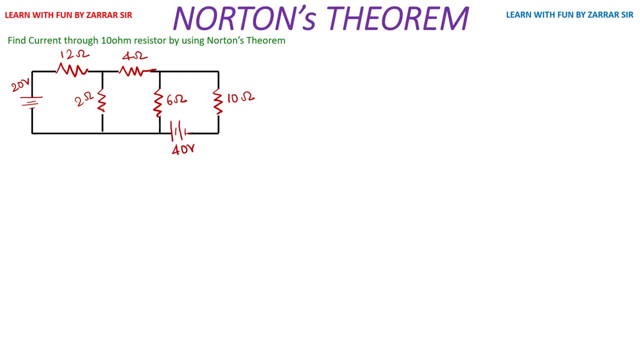 So this is a circuit of which this is the 10 ohm resistor that we need to find using Norton theorem. okay, so the first step of Norton theorem is step number one: remove the resistance 10 ohm and short the path. okay, so you need to remove the resistance 10 ohm, you have to short the path. 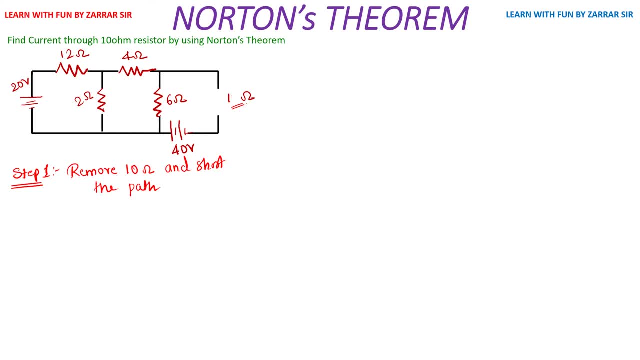 so i'll remove this 10 ohm resistance, okay, and we'll use this 10 ohm resistor. two volts is the end of the step of Norton theorem, so I'll short this part, okay. so this is the first step. you need to remove the 10 ohm resistance which we need to find. 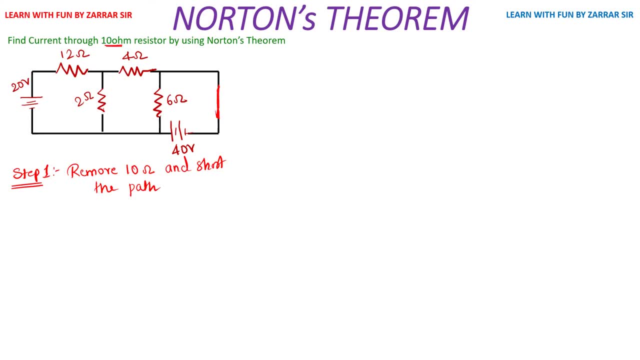 current across 10 ohm resistance. you need to remove that resistance. so this is the first part. now you have to find current across the 10 ohm resistance. so this is I n the current across 10 ohm resistance. so how I will find out is I. 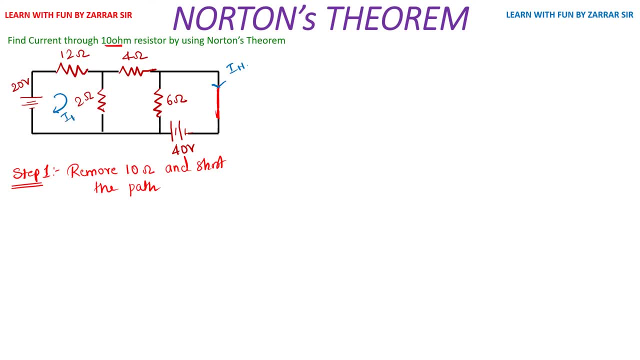 will apply KVL in loop 1, I 1, I 2 and I 3, and I have already given you a shortcut video of how to find KVL across I 1, I 2 and I 3 or across the loop. so we'll find out applying KVL at loop 1. KVL at loop 1. if you apply KVL at loop. 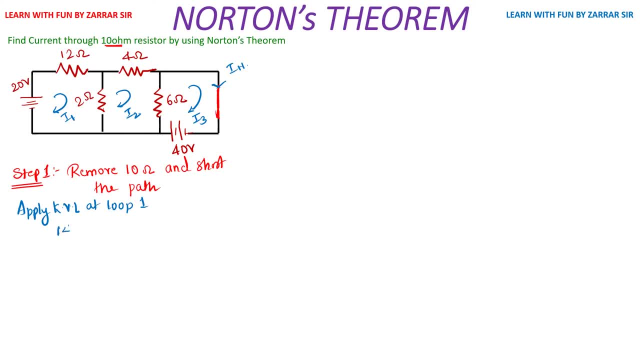 1. 12 plus 2 is 14 I 1. right, I don't need to discuss the shortcut again. you can refer the previous video. 12 plus 2 is 14 I 1. this 2 ohm is in second loop, so I'll write. 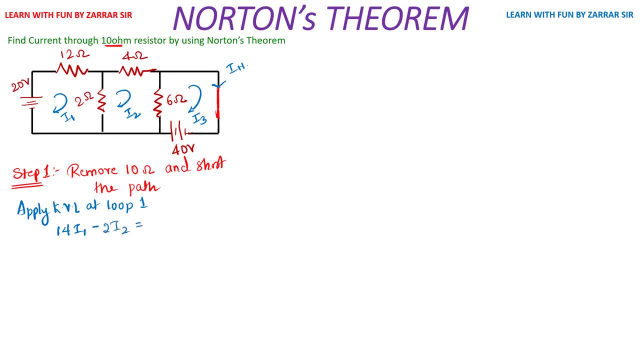 minus 2, I 2 and since there is no current I 3 over here, so I 3 will not be there and you are moving from negative potential to positive potential. you need to write positive 20 volt, okay, so this is your KVL at loop 1. similarly, I'll. 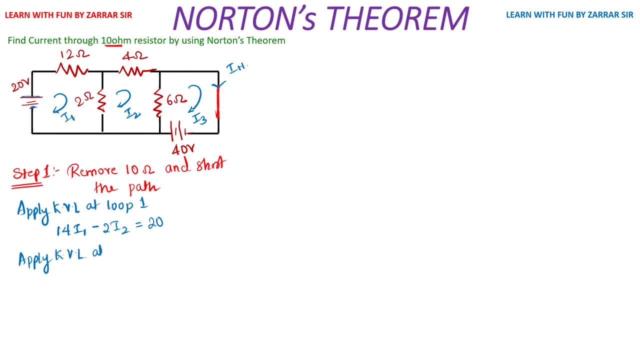 apply KVL at loop 2. okay, let's hit thisself here. so let's see, let's say I want to apply 12 ohm, I 2. right, I will write 12 ohm ist in first loop, KVL at loop 2. so once you apply KVL at loop 2, 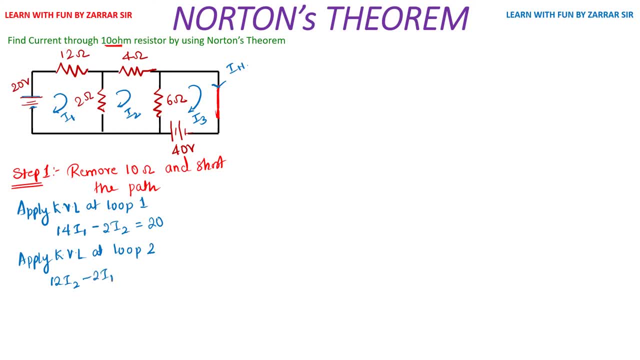 4 plus 6, 10, 10 plus 2 is 12, so I'll get 12 I 2- I'm using the shortcut. 2 ohm resistor is in first loop. I'll write minus 2 I 1. 6 ohm resister is in third. 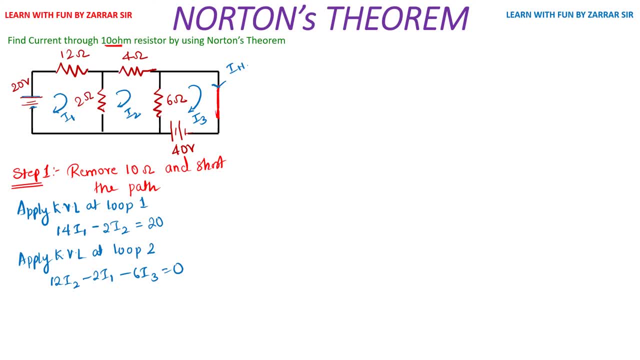 no voltage in the second loop. so this is the kvl at loop 2 and the final kvl apply kvl at loop 3. so if i apply kvl at loop 3, what will happen? 6 is the only resistance of at loop 3. so 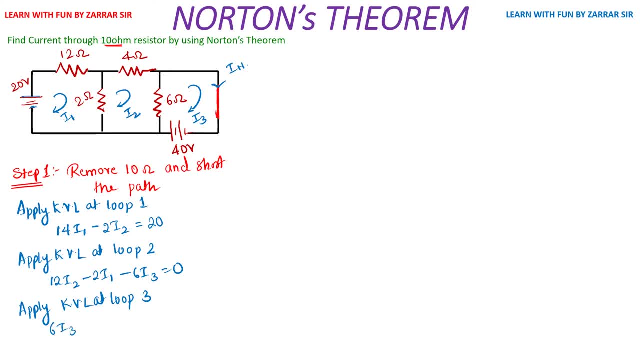 i3, 6 i3. this 6 ohm is also in loop 2, so minus 6 i2. and now i have a voltage 40 volts and i'm moving from negative potential to positive potential, so i'll write positive 40. so these: 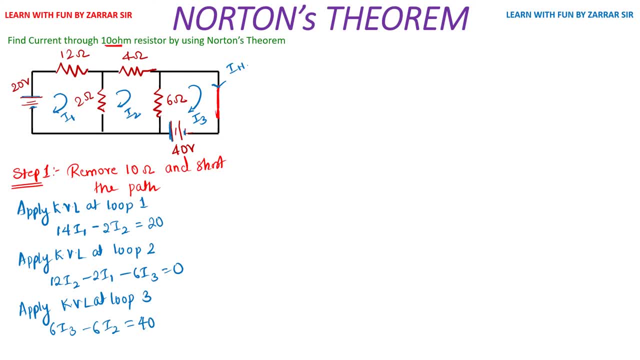 are the three. i would say these are the three total equation of all the three loops. so i got the three equation. once you solve this three equation in the calculator using simultaneous equation, you will get the value of i1, i2 and i3. i have already solved for you so that your time 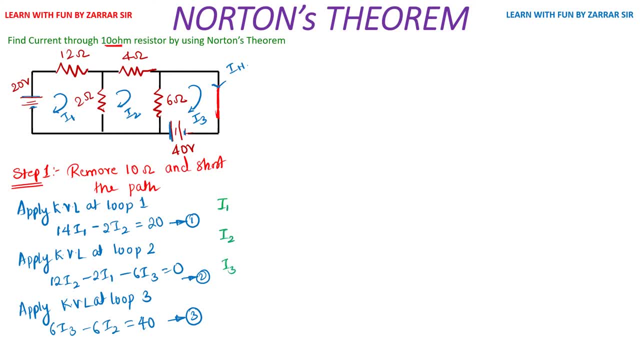 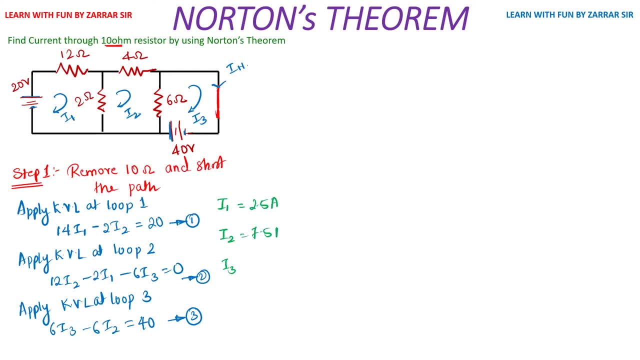 okay, i2 has 7.5 ampere, you can check it also. and i3, which is my norton current, you will get 14 point 14.166. okay, so this is your i3. so you have got all the three uh current, that is, 2.5 and 7.5 and 14.6. as you can see, the norton current i? n and. 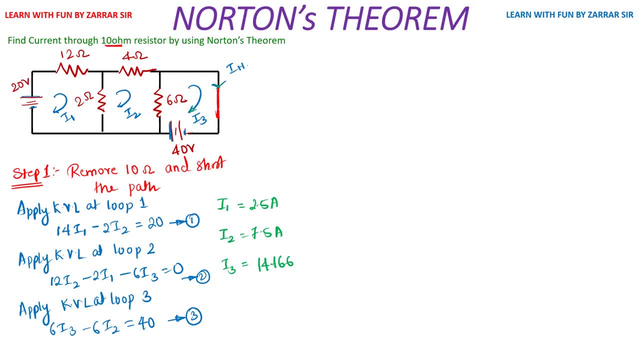 i3 has same direction, so i can directly write: i: n is equal to, i3 is equal to 14.166. okay, so this is my final norton current now, as you have already got the norton current now the second step over here is you have to find the norton resistance. how to find norton resistance? 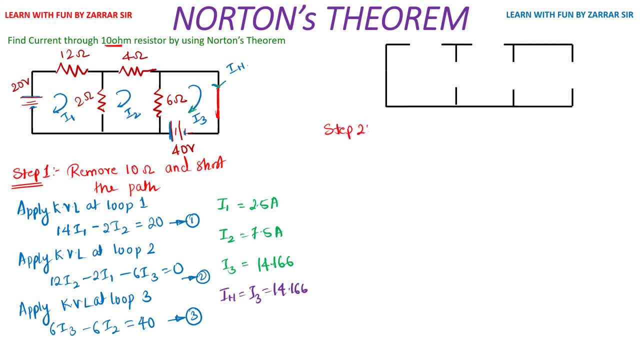 i have already drawn a circuit again. so step two is norton resistance. so finding norton resistance is very simple, or thevenian resistance, any resistance that you need to find thevenian or norton, you have to short all the voltage sources and open current sources. so this is the first voltage source. as you can see, the 20 volt is over. 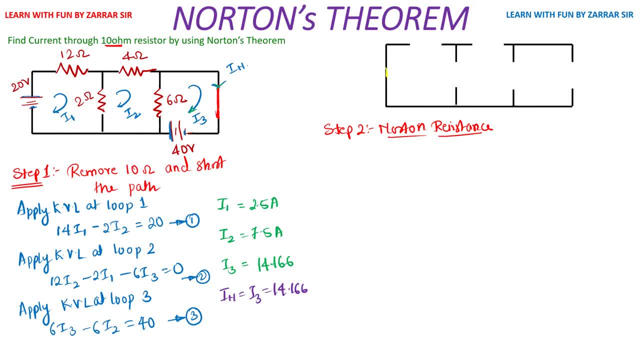 here. so i've shorted the 20 volt. okay, this is 20 volt which is shorted, and this is the 40 volt over here which will get them shorted. so i'm going to short it now. i'm going to short it now. i'm going to. 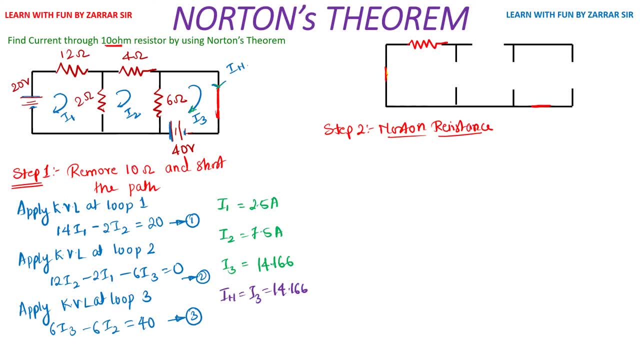 give you all the voltage sources and i'm going to write this in to the norton current i, n and i'm going to show you the norton voltage source. as you have already seen, this is a very simple circuit. it's just a very simple circuit. you come with only few resistances. the first resistance. 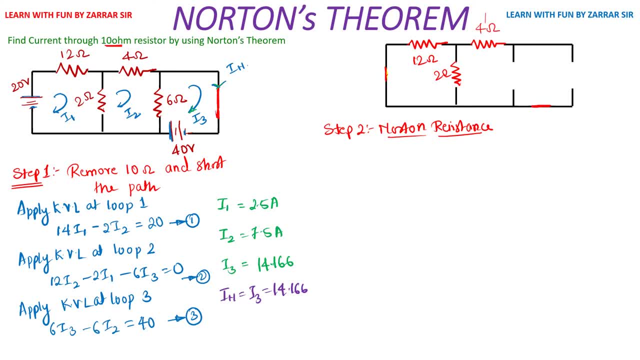 will be over here: 12 ohm. the second resistance is over here, which is two ohm. another third resistance is over here, which is four ohm. four ohm. now we have one more resistance over here, rn. so this is your voltage. i mean, this is your resistance. this is the path from which you will. 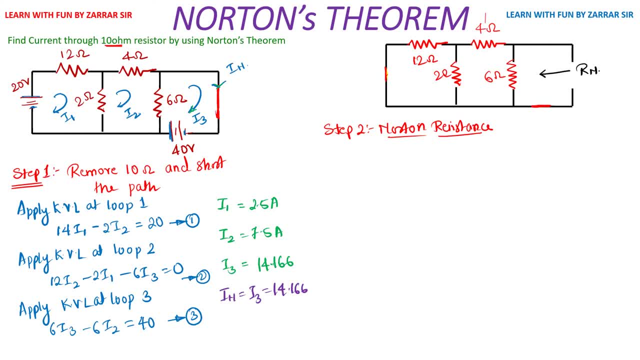 be seeing norton resistance. i'll give you the trick over here also how to calculate norton resistance. so you have to enter from here and go to the end point. from n you need to take all the resistance and come back to this original point. so if i enter from here, 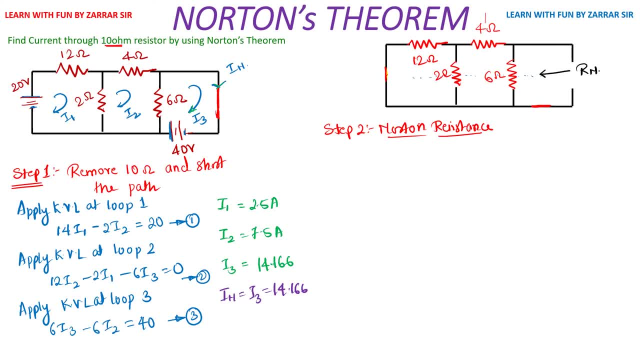 if i enter from here, i i reach at a point where i get 12 ohm in parallel. as you can see, 12 and 2 are connected at both the terminal, so can i write 12 plus 2, so my final rn will be equal to 12, okay. 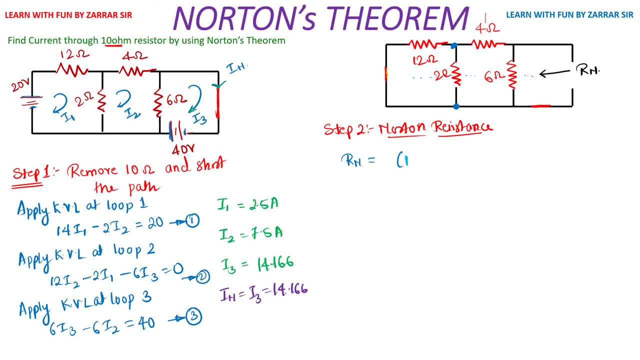 my final rn will be 12 in parallel bit 2. okay, so this is the first part, 12 parallel bit. now, once you get 12 parallel with 2, this circuit gets complete. this resistance get completed and you can see this resistance is in series with 4 ohm, so i'll write plus 4 ohm. okay, so you have this resistance, which is: 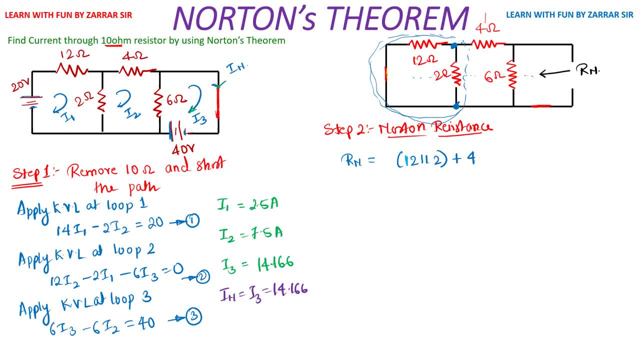 in series with 4 ohm. once you have added 4 ohm now you can see this whole resistance which i'm talking about. is this 4 ohm and this resistance is done, and this all are connected with 6 ohm in parallel configuration. so i'll what i'll do is i'll write parallel 6 ohm, okay, so this is the final value. 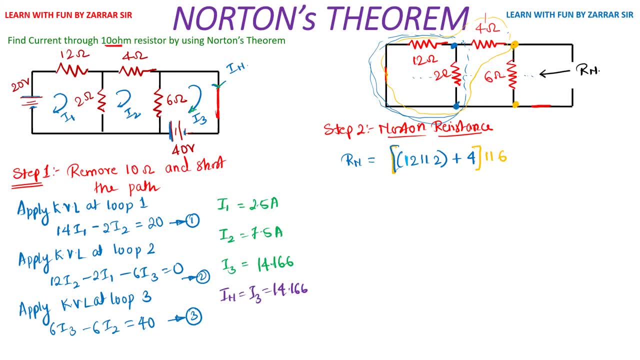 the final resistance calculation you'll write parallel with 6 ohm. and once you have written parallel with 6 ohm, the final value turns out to be: if you calculate this, you know how to calculate- it get 2.926 ohm. so the first step is to remove 10 ohm and short the path and calculate in and calculate. 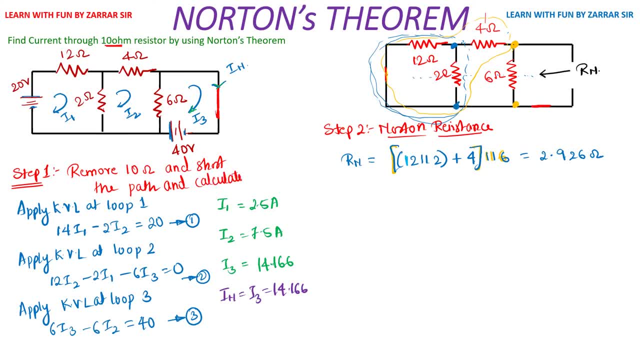 in. so first you need to calculate, in the second step is norton resistance, and now the final step. so the final step is this circuit, which is norton circuit. so step number three, norton circuit. now see how to calculate its current across 10 ohm using norton's theorem. 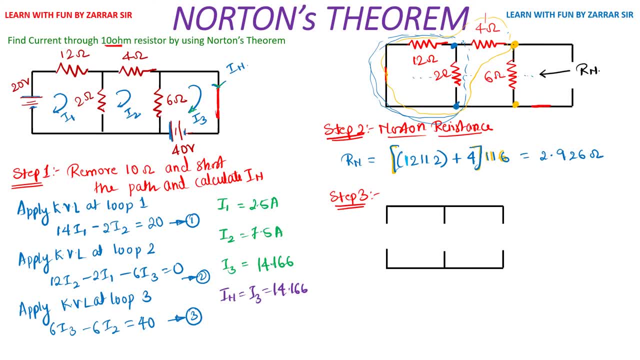 so this is final norton circuit. what i'll do is the current that we have got. it is you have to draw it over here. we'll write it as in: okay, the resistance what you get, you'll write it as two point two: 926 ohm, and the final resistance that we removed in the start from here was 10 kilo ohms, so you'll 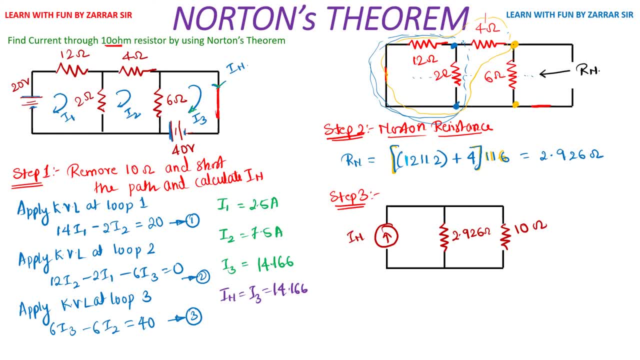 write 10 kilo ohm and then- it's a very small step- you have to calculate current across here. so let's name this i1 and let's name this i2, and you know how to calculate i2 using current division rule. okay, so using current division rule and in is nothing but. 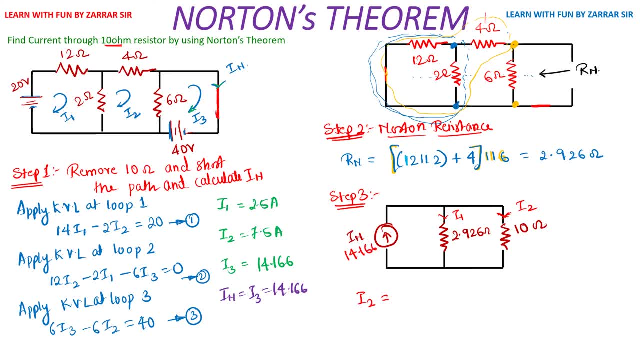 your total current, 14.166. so you know how to calculate it is. it's very simple. if you need to calculate current across this resistance, you have to take its opposite resistance. okay, uh, 2.926 upon total resistance. 2.9 plus 10 is 12.926 multiplied by total current, which is 14.166. and once you solve, 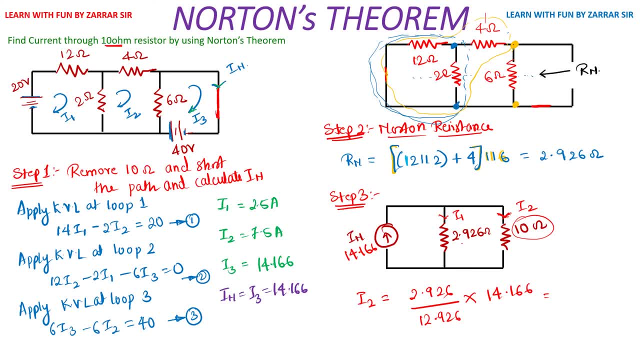 this, you get the value, as once you solve this in the calculator, you'll get the value of 3.206 ampere, which is your final resistance. so this thing is important and if you have any problems with this, which is your final current across 10 ohm resistor. so this is the way we need. we draw norton serum. 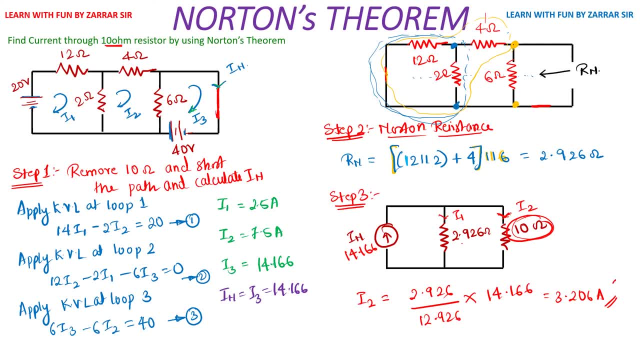 or we solve circuit using norton serum. so the current direction will be downwards. it's very simple to see: the current will be coming in the downward direction. so there are three steps, guys. the first step is you have to remove 10 ohm resistance and short the path and calculate in. 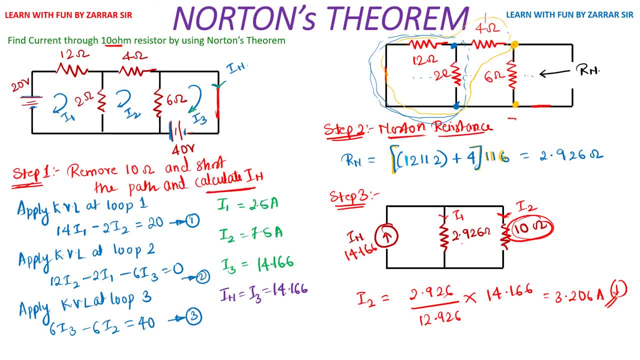 the second step is you need to calculate norton resistance. while calculating norton resistance, make sure you short the voltage source. okay, since this problem doesn't co contain any current source. so you have to short the voltage source and open the current source. okay, open current source. 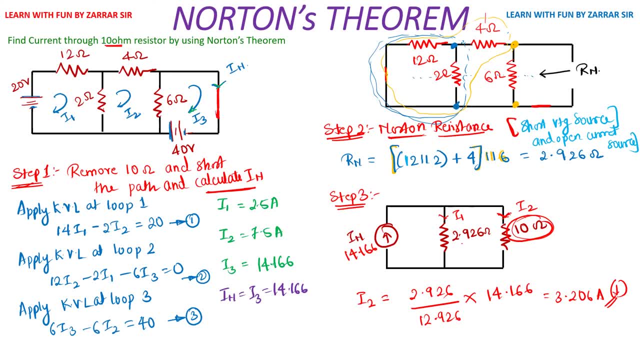 and you'll get the resistance which is rn. so you can solve this. this is very simple. you first calculate parallel resistance 12, parallel two, you add with four and the final resistance value parallel to 6, and you know the way should enter and reach at the end. final points from. 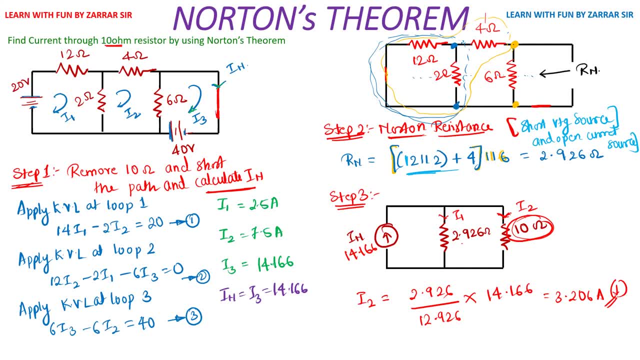 final point. you can calculate all the resistance and come back. so this is the way to calculate rn once you get rn and in. so once you get in and rn, this is the final circuit. that is, you have one in and rn, so i'll write in: you have rn and then the load that you have removed, which was 10 ohm. 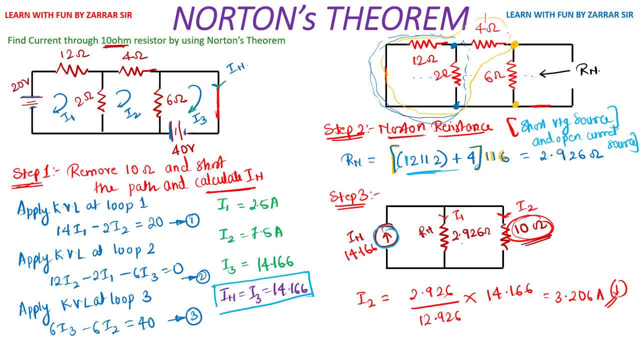 you will draw at the end. so remember one important concept in Thevenin or Norton, whenever you are asked to find a current across any resistance, you will remove that resistance and you will bring that resistance at the end okay, and you will use that resistance at the.